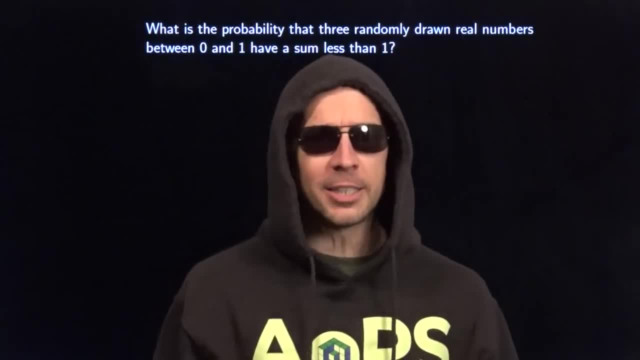 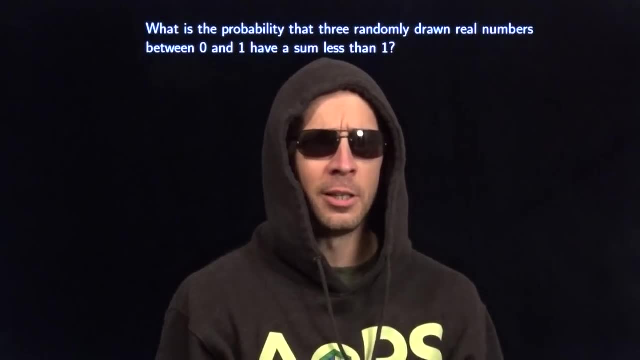 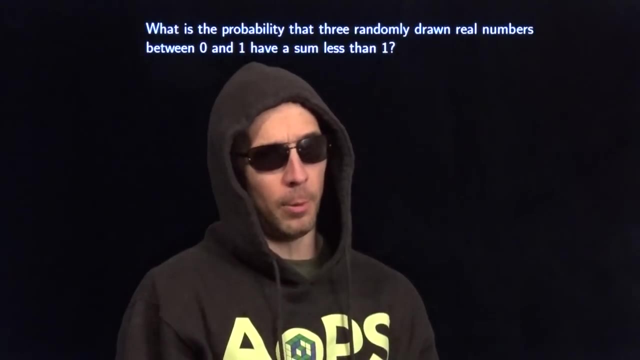 his face. just he got all excited. He got all excited And then he said I got to go get Harvey And he ran out of the room. That kind of confused me because I don't know who Harvey is. But while he's off finding that Harvey dude, I'm going to solve this problem Now. here's. 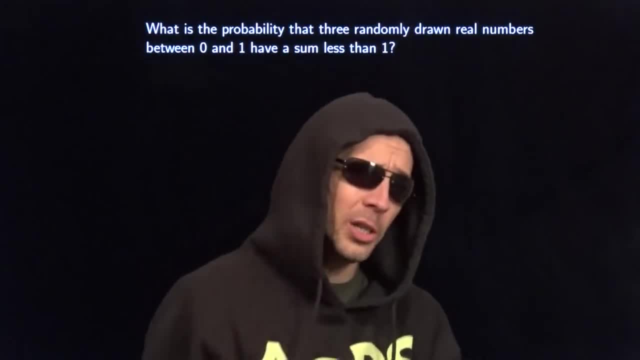 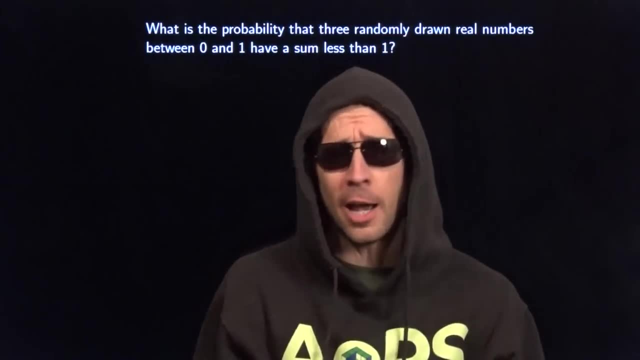 how I'm going to start. I'm going to start by forgetting about that. three randomly drawn numbers. I'm going to start off with two, because maybe you haven't ever seen anything like this before. So three numbers kind of freaks you out. Let's start with two. We're going. 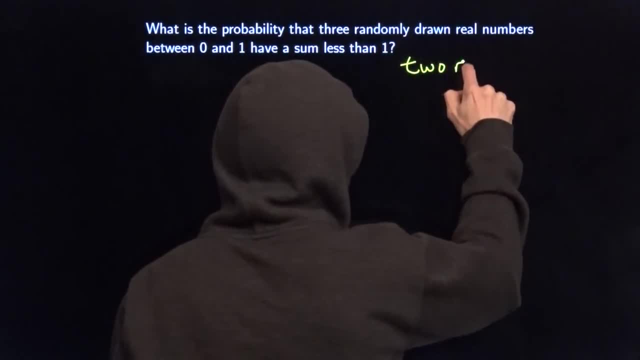 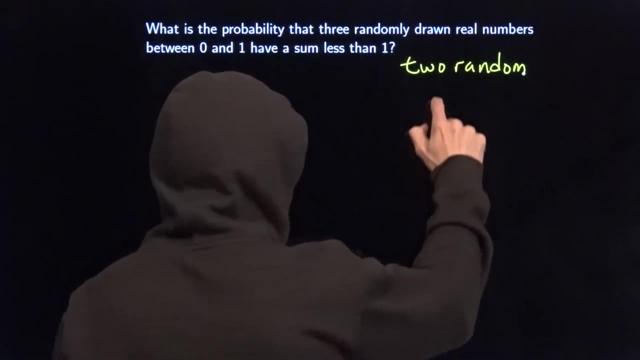 to start with just two randomly drawn numbers between 0 and 1.. Now I'm going to call those numbers x and y. So we're going to take an x and y randomly drawn between 0 and 1.. Now, as soon as we say 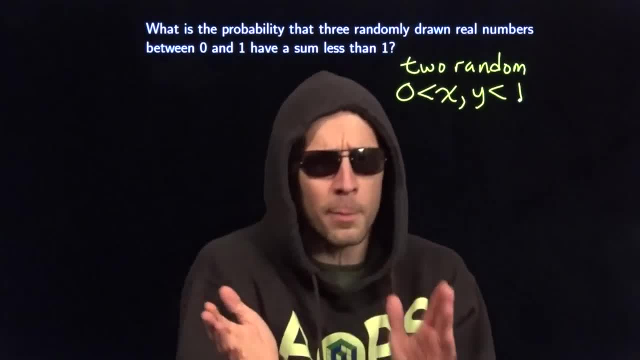 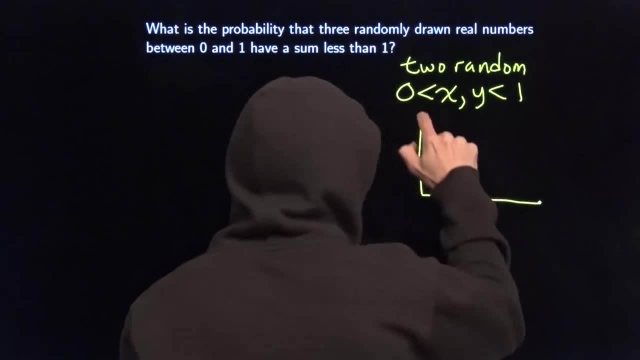 x and y, we start thinking: where have we seen x and y, two numbers before Coordinate plane? So we're going to draw a picture of what's going on here, And that's what I like to do when I have infinitely many possibilities, because geometry has great tools for measuring. 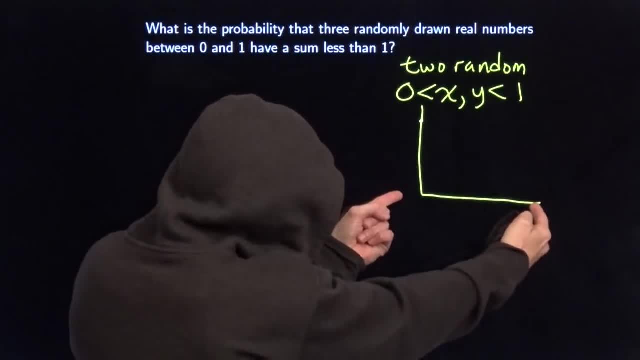 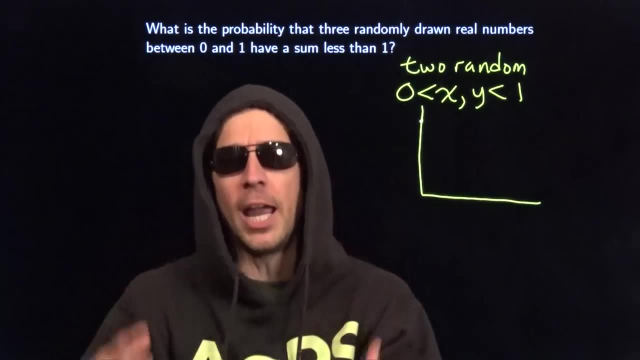 infinite sets of points. We can use length. Just this little segment right here, right there It's got infinitely many possibilities, points, but we can measure it, We can find its length And we also have area. So let's try to. 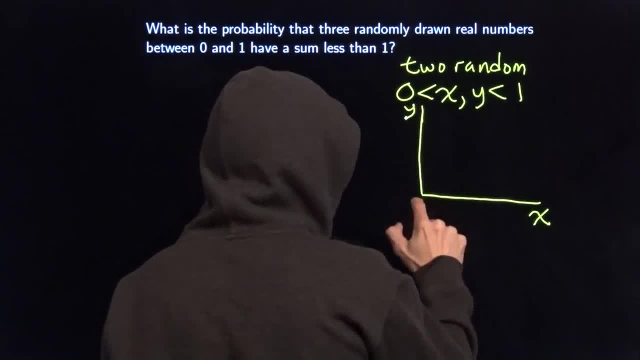 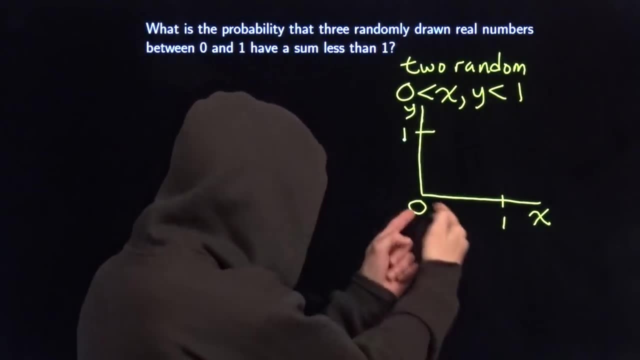 use that. Put x here, put y here. We're going to say this is zero, We'll call this one, We'll call this one And this. x and y are between zero and one. That means x is between zero and one. That. 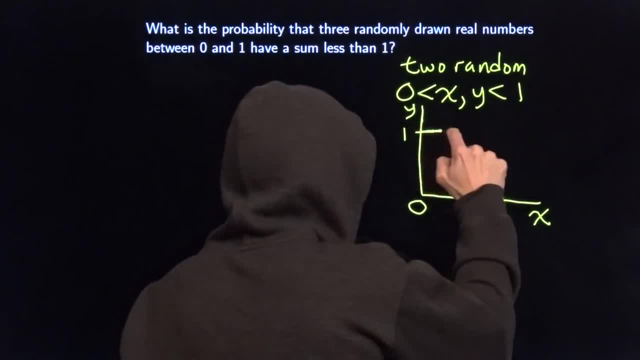 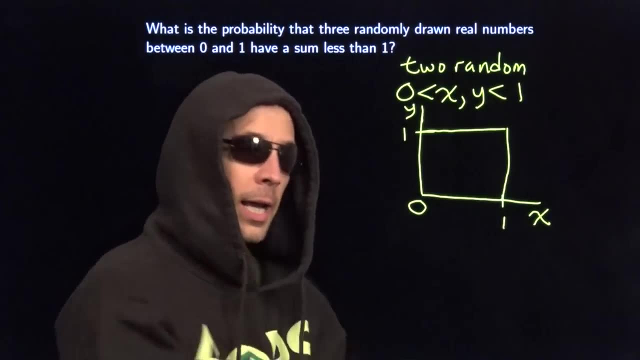 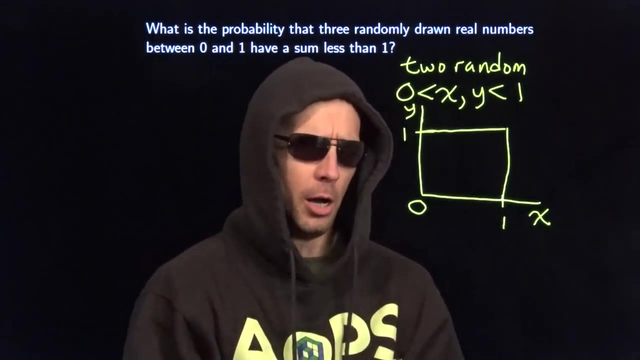 means y is between zero and one, That means the combination of x and y. that represents a point that is in this square, And we can measure that square with area. That square has area one. So we found the area of our possible region. It's one. Well, now, what's our desired region? We want the. 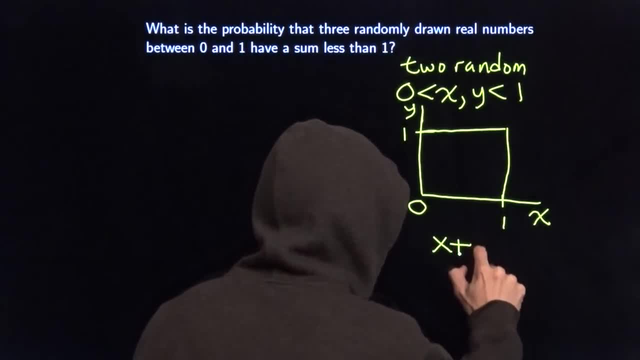 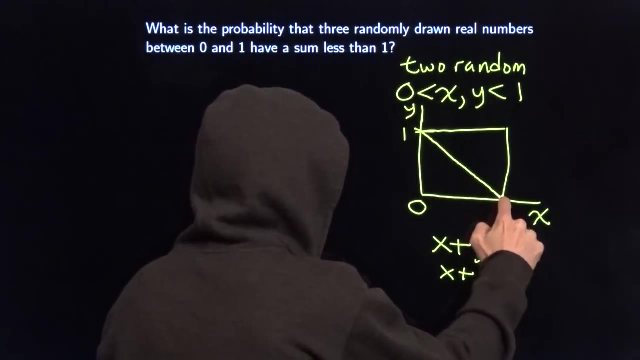 sum of these numbers to be less than one. We want x plus y less than one, But where's that in this picture? We'll start off with: x plus y equals one. X plus y equals one. That's just a line. That's this line right here. X plus y less than one. That's everything below. 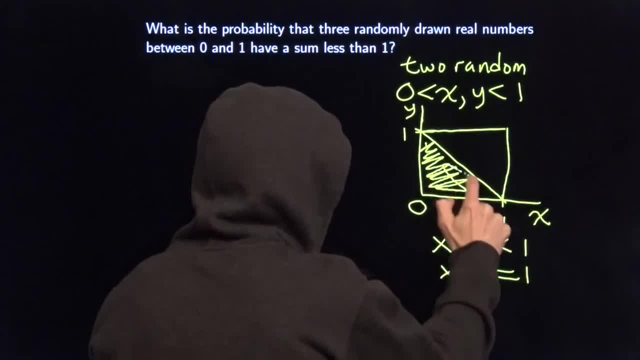 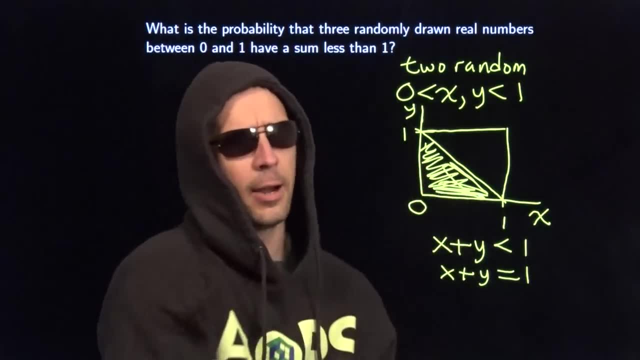 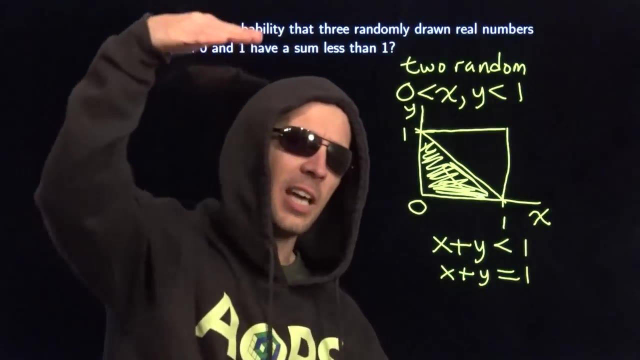 the line. It's everything down here. So our desired region is this little triangle right here, This right triangle with legs of length. one Its area is one times one. You take half of that, you get one half. That's our desired region area. Take our desired area, divide by our possible. 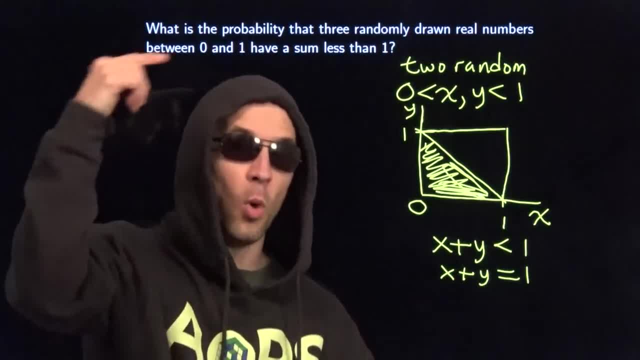 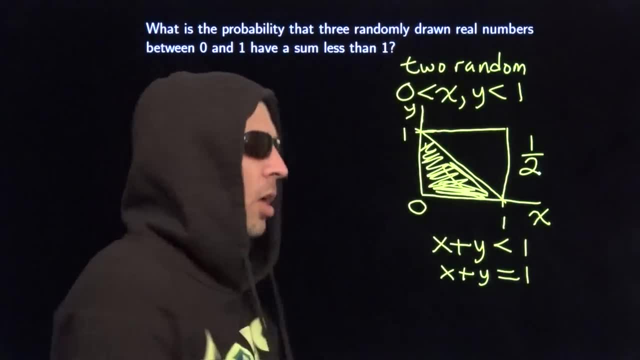 area, That's the whole square, You get one half Divided by one is one half, So the probability over here is a half. Now we're ready to think about three randomly drawn numbers. Now, when we were tackling two numbers, we had x, We had y, But we've 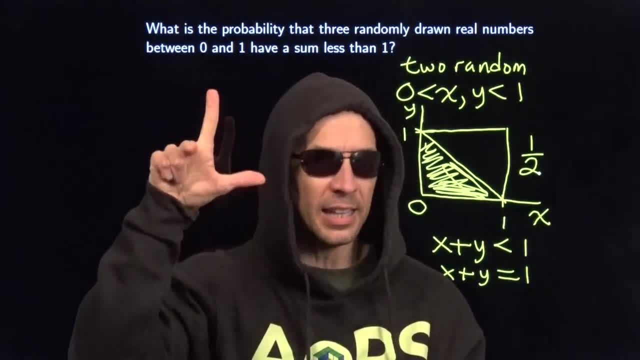 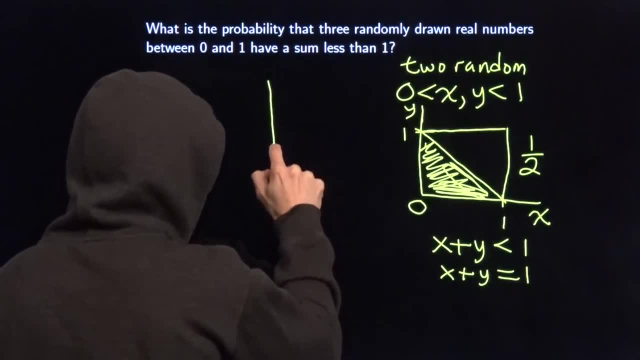 got a third number now, so we've got z, Just like that. That's right. We're still going to be working with coordinates here, But now we're going 3D. Let's go ahead and draw a picture. We've still got our x. 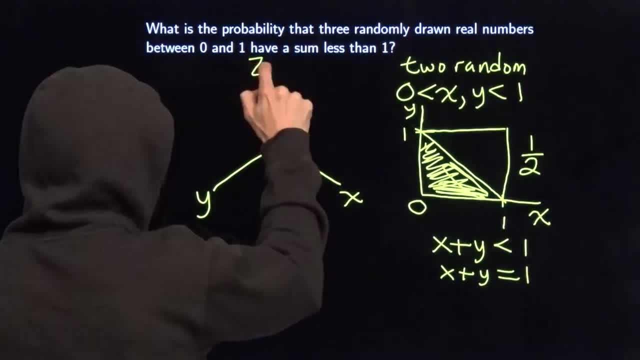 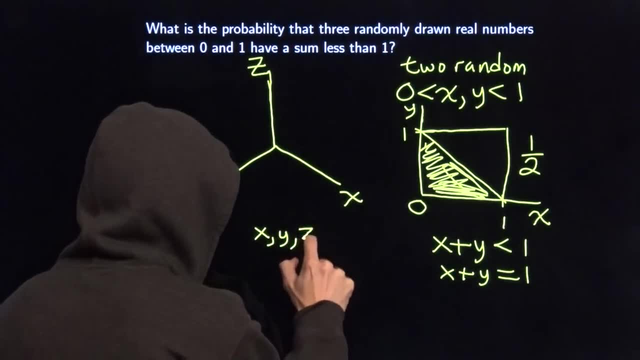 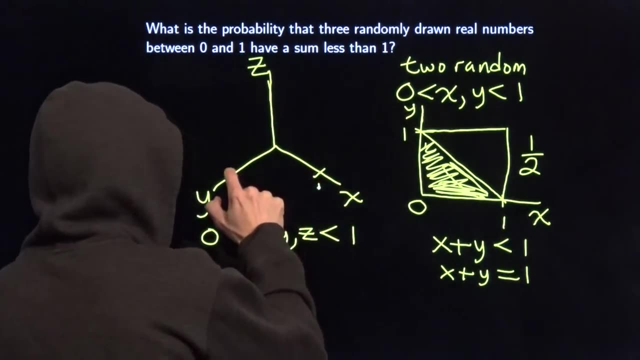 our y, but now we've got a z And we still want these three numbers, this x, y and z. We want them all to be between zero and one, So we'll call this one. We'll call this one. We'll put one right up there. 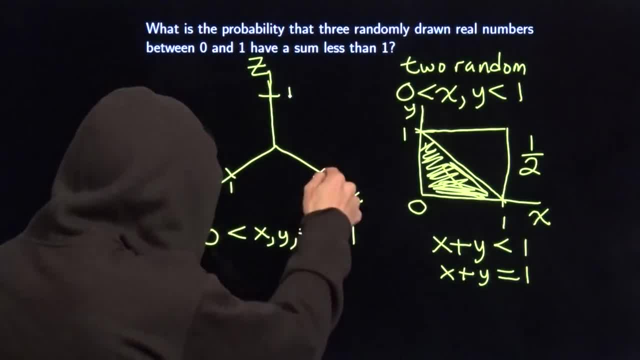 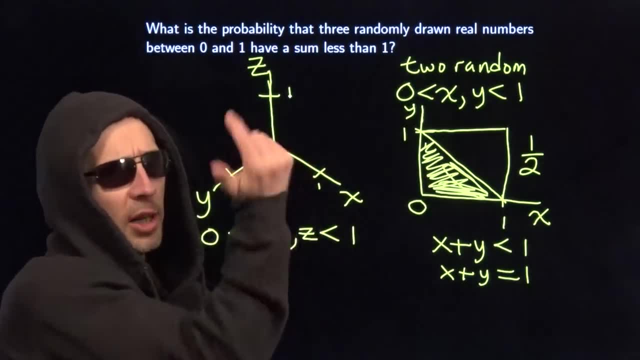 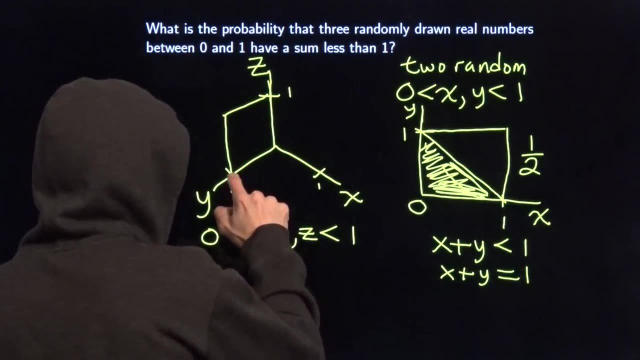 We need x, y and z, all to be between zero and one. So we need x between zero and one, Y between zero and one, Z between zero and one. We're in 3D Now we've got a cube. This is our possible region. This is the cube of all points. 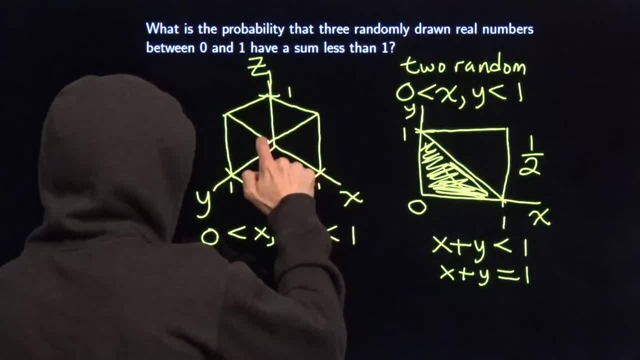 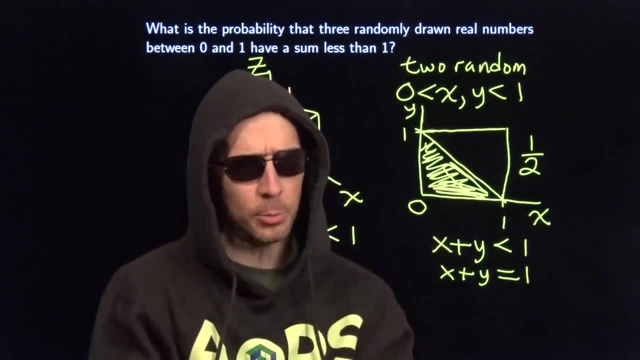 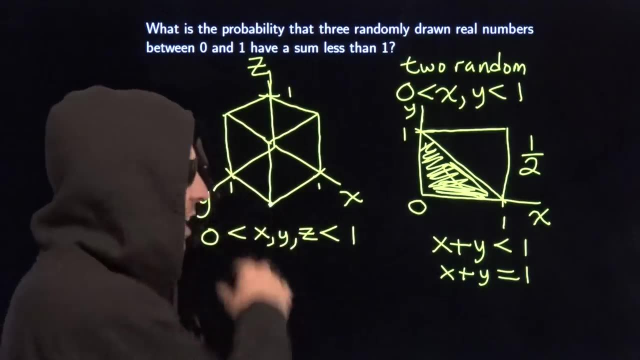 for which x, y and z are all between zero and one. Now, over here, we used area to measure our possible region. Here we're in 3D. Now we're using volume, The volume of this cube. well, all the sides, all the edges. 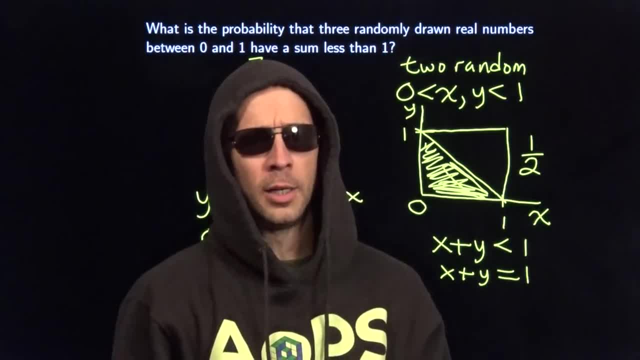 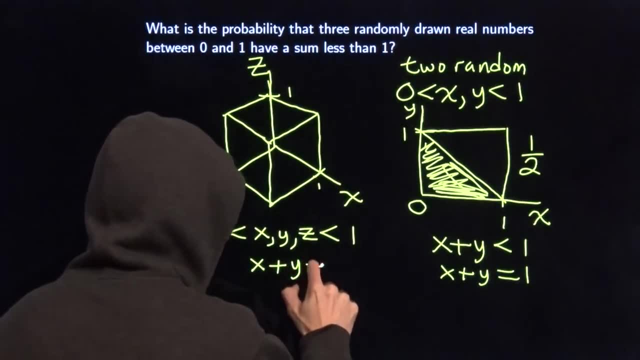 that have length one, the volume of that cube is one. So now we gotta deal with what's the desired region. Where do we have x plus y plus z Less than one? Where does that happen? Let's start off with x plus y plus z equals one. 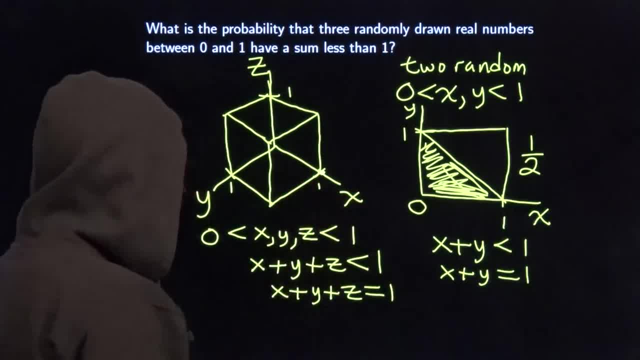 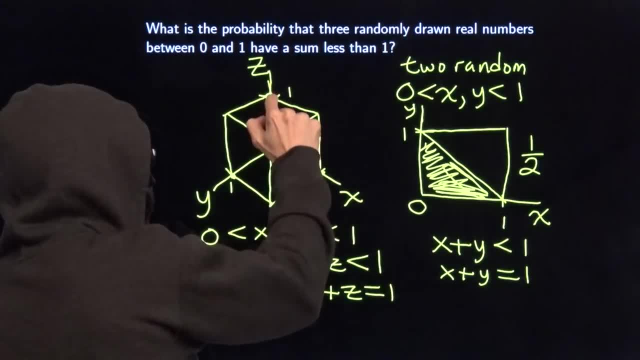 x is one and y and z are zero, We're right there. If y is one and x and z are zero, We're right over there. and if x and y are 0, then z is 1.. It's right up there. 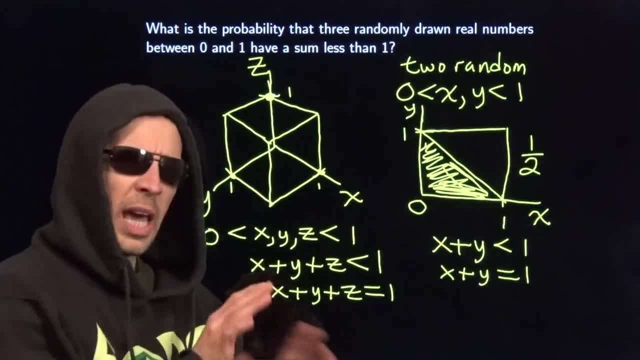 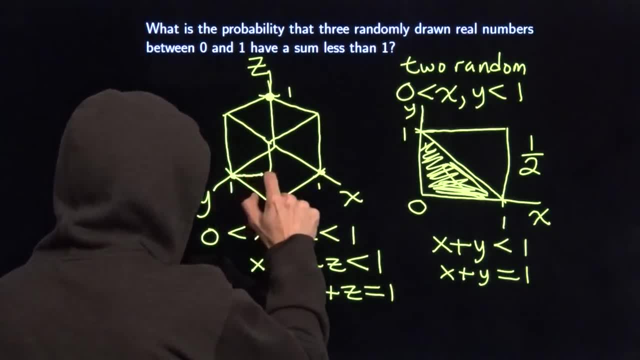 Well, now let's take a look at what happens when z is 0, and x and y can vary, but x plus y has to equal 1.. Well, that's a line. We had that right over there. It's this line right there, and that's where z is 0, so we're down here in the xy plane. 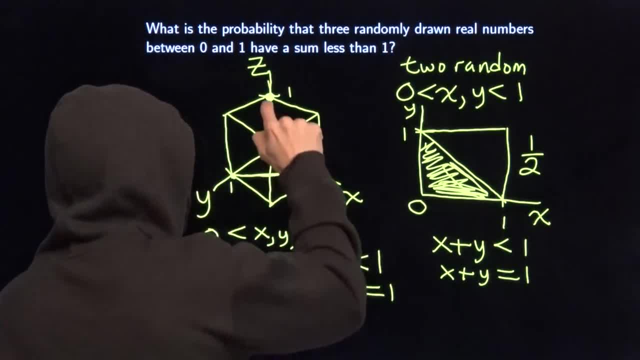 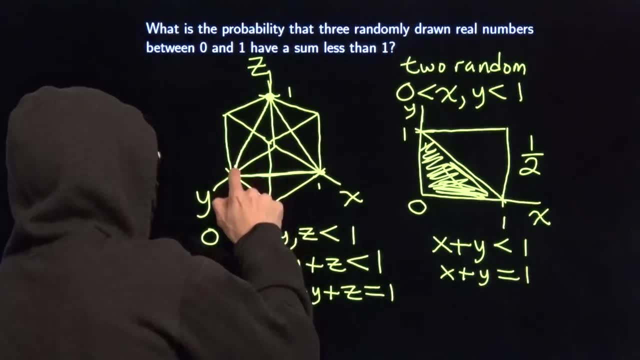 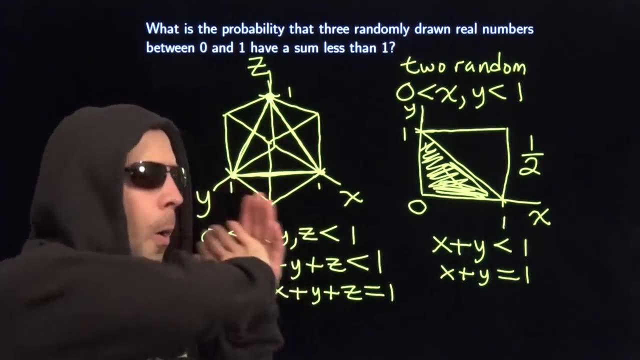 and x plus y equals 1.. And then when y is 0, we have x plus z has to be 1.. And then, when x is 0, y plus z has to be 1.. We build this triangle right here, and this triangle is part of a whole plane where x 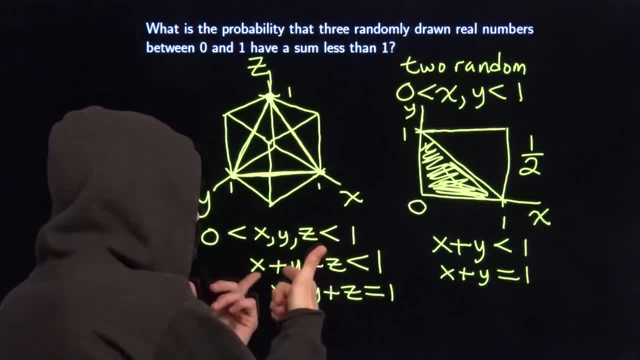 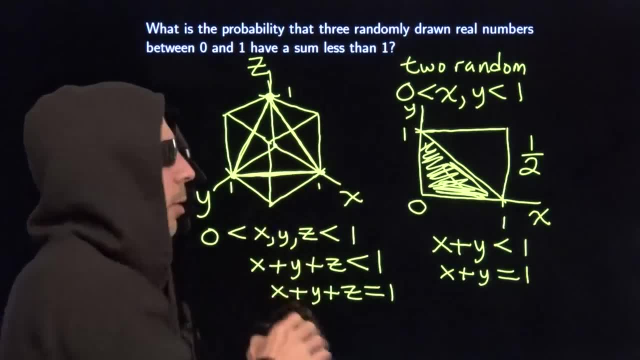 plus y plus z equals 1, but we want x plus y plus z to be less than 1, so we got to go below this plane, We got to go back towards the origin, back there where they're all 0, so we want everything. 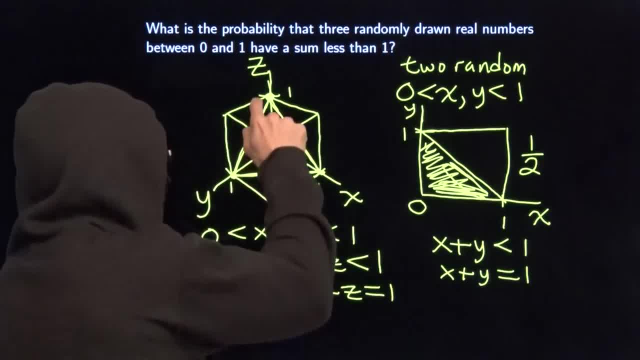 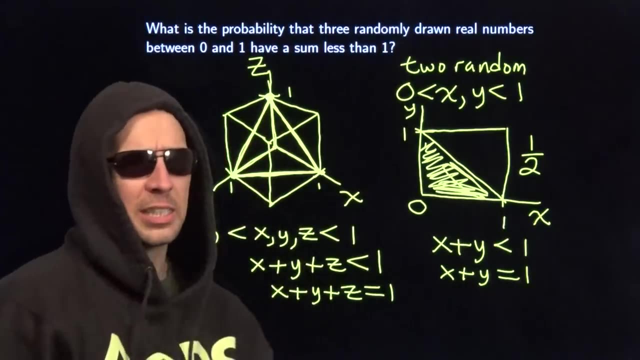 under there. That's our desired region. It's got 0.. 0. These three sides of this triangle as edges, and then back here these parts of the z axis, the y axis and the x axis. This is our desired region. 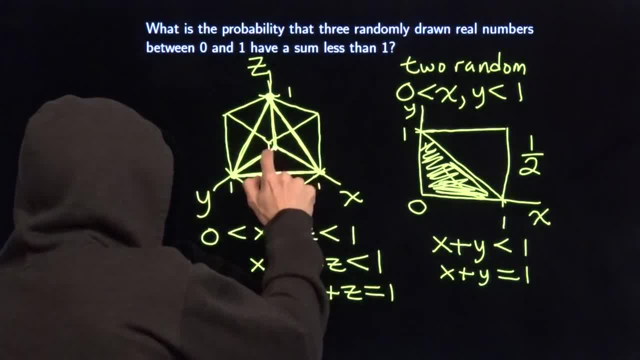 It's a pyramid. It's a pyramid. The base is right here. It's a right triangle with the legs of length 1, so its area is 1 half. The height of this pyramid is going right up here. That height is 1.. 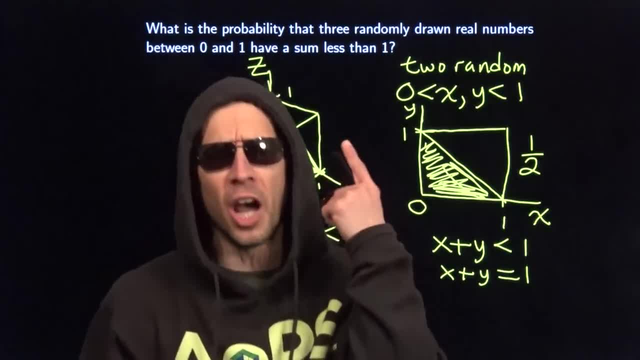 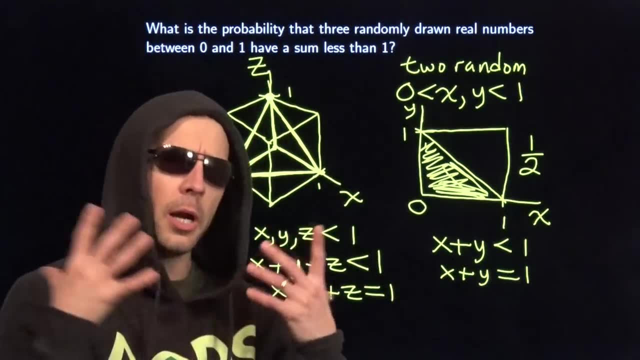 The volume of that pyramid. we take the area, that 1 half. we multiply by the height, that's 1, and then we take 1 third of that product. That gives us 1 sixth. So our desired volume there is 1 sixth out of the possible volume of 1, 1 sixth divided. 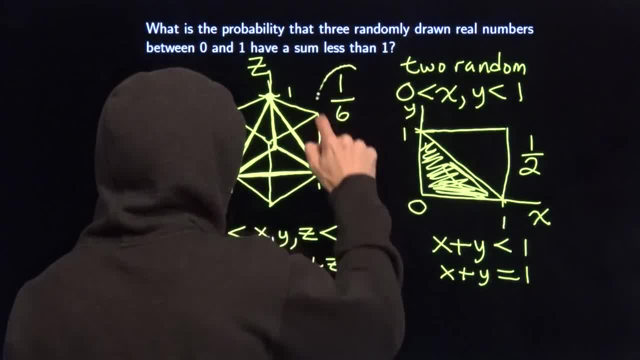 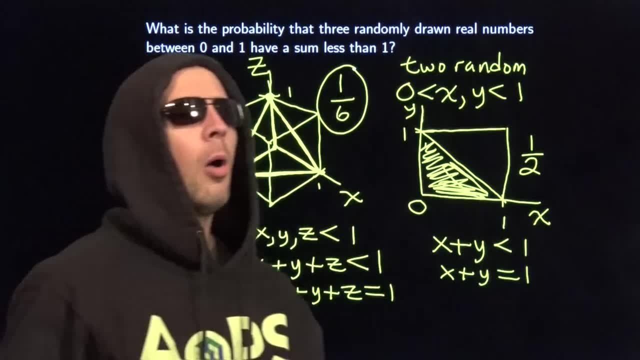 by 1.. That gives us the probability of 1- sixth, and we've used geometry to solve this probability problem. Hey, oh, hey, man, You coming here. Help me out here, I'm already done. Oh, what's your name, man?